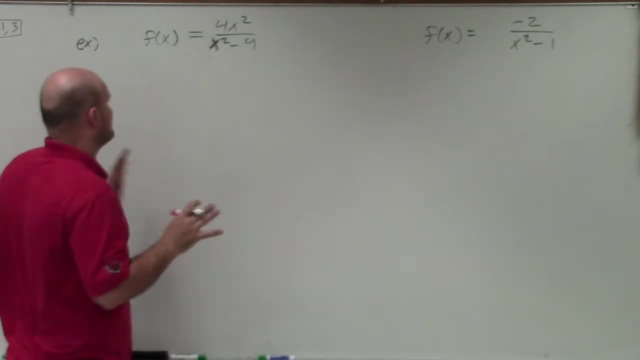 by a little bit quicker. So if you need to kind of rewind or so forth, please do so. So the first thing we want to do, though, is find our symmetry. So remember to find symmetry. basically, what we're going to do is we're going to plug in f of negative x. 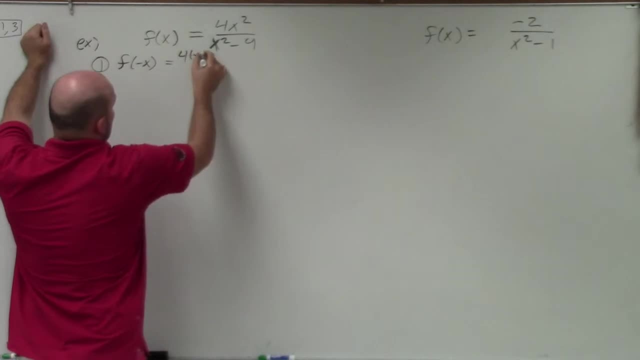 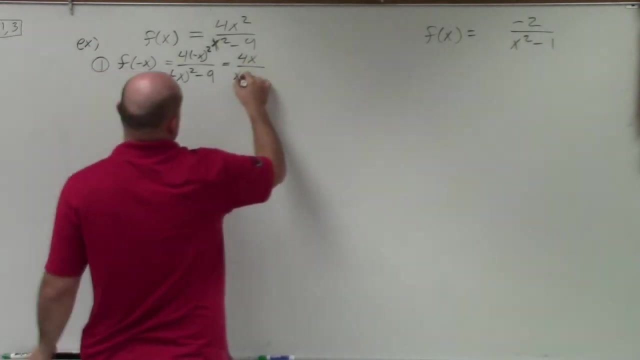 And if we obtain the exact same function back, then we have symmetry about the y-axis. If we obtain the negation of the function, then we have symmetrical of about the origin. So negative: x squared is just x squared And x squared is just x squared. So you can notice. 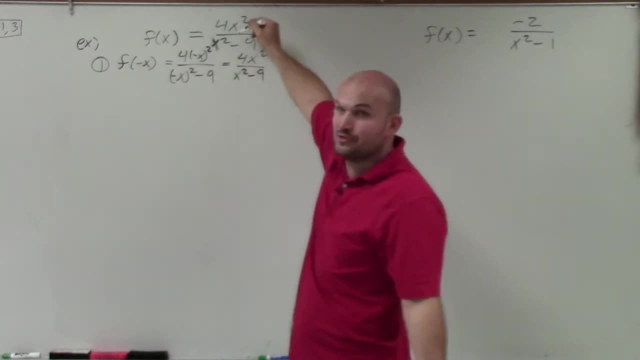 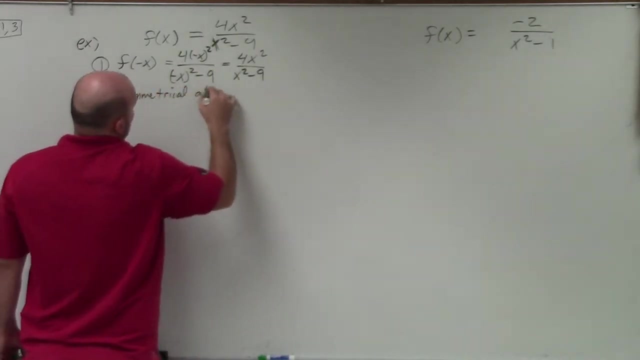 that when I plug in negative x, that doesn't change the function. I actually revert back to my original function. So therefore this is symmetrical about the y-axis. So again, why is this so important? So when it becomes time defined. 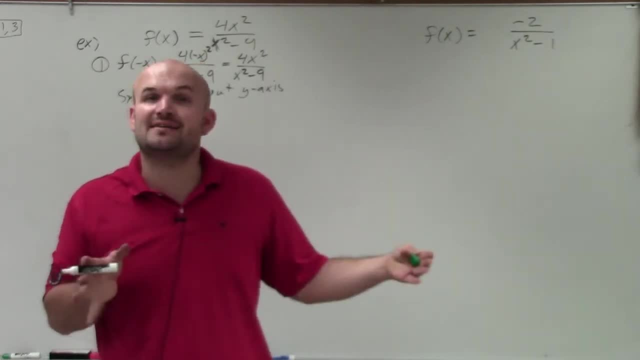 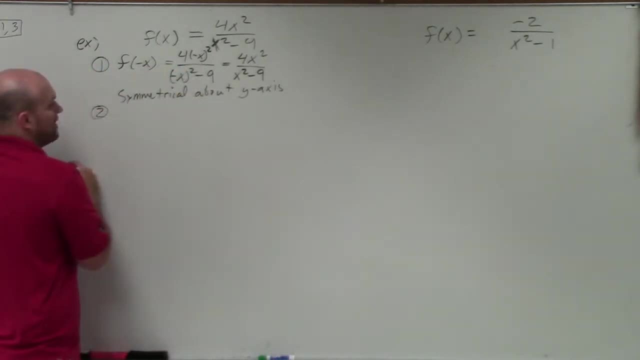 Determine the points that we're going to plot. We only need to pick the points on one side of the y-axis and then we can reflect it over to the other side. All right, the next step is to find the x and the y-intercepts. So basically, remember, the y-intercept is: 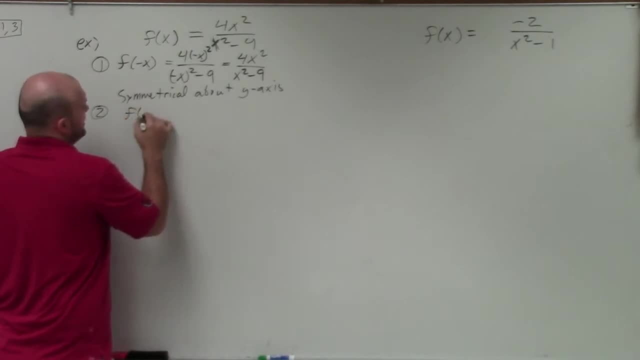 going to be when x equals 0.. So basically, I'm just going to plug in 0 in for x. So that's going to leave me with 4 times 0 squared divided by 0 squared minus 9.. Well, this 0 squared. 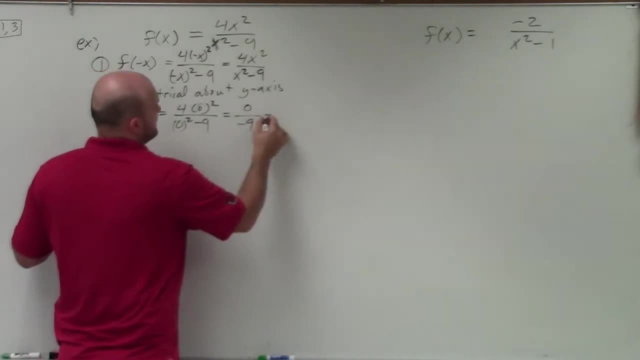 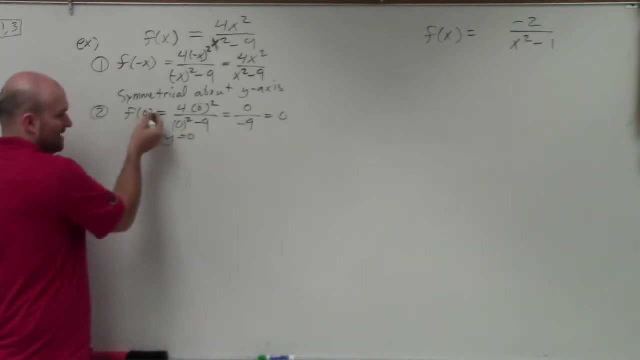 0 times 4 is 0, over 0 squared is 0 minus 9. And therefore that equals 0.. So therefore the y-intercept is just at: y equals 0 when x equals 0.. Step number 3 is to find the x-intercept. 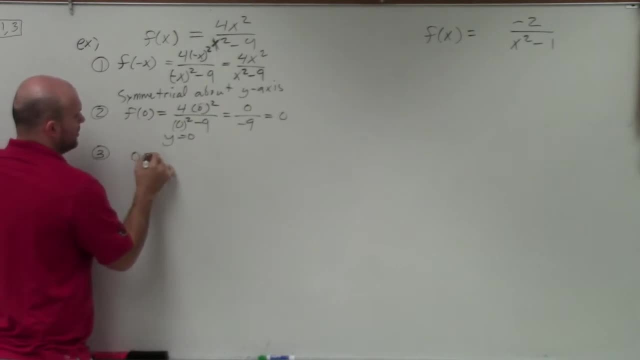 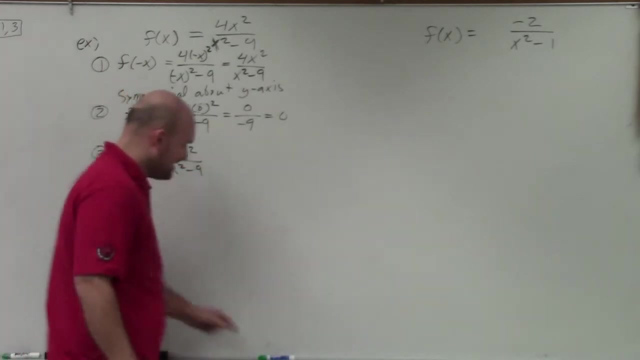 The x-intercept is when the whole f of x is equal to 0, or your whole y value is equal to 0. So therefore I have 4x squared divided by x squared minus 9.. I'll show again this because it confuses students all the time If you need to solve for x in this equation. 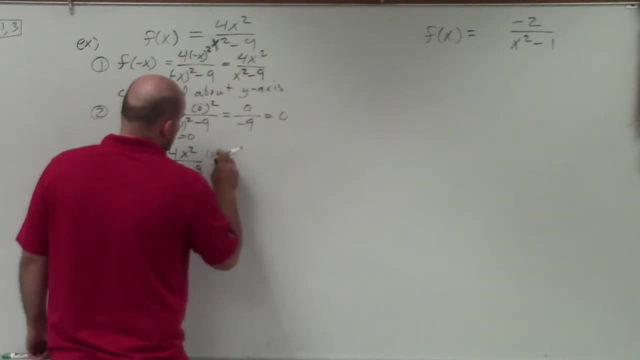 we've got to get x squared minus 9 off the denominator. So the way to do that is to multiply by the reciprocal. It doesn't matter what I multiply over here. So therefore, now those divide out, This multiplies to give you 0.. So you're left with 0 equals 4x squared. So 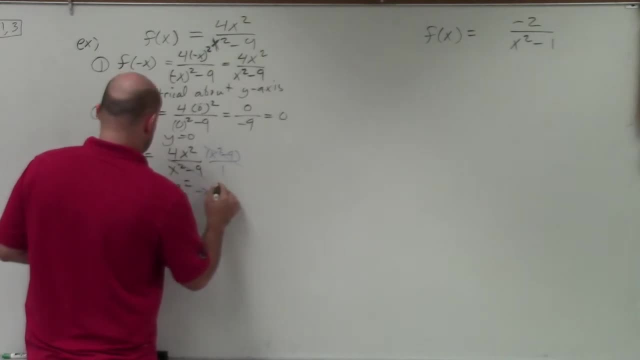 you divide by 4. And you get 0 equals x squared. Take the square root, Take the square root And you get x equals 0.. So I now have- So I know it's the math, I know it's symmetrical- about the y-axis: I have a y-intercept at 0.. I have an x-intercept. 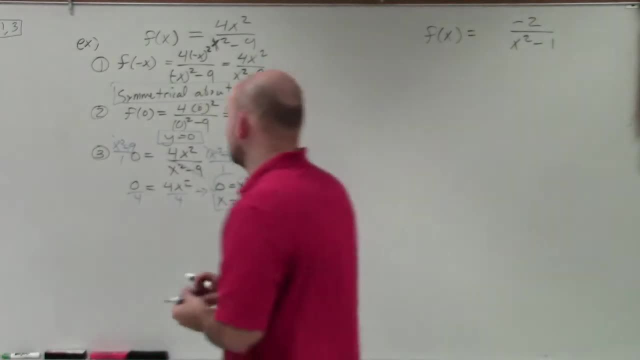 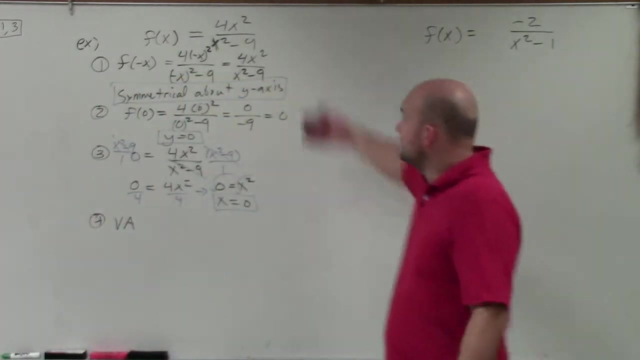 at 0.. The only thing we need to do is now determine our vertical and our horizontal asymptotes. So step number 4, vertical asymptotes- Remember, the vertical asymptotes is basically when the denominator equals 0. So we go back to our denominator and say, all right, I'm going. 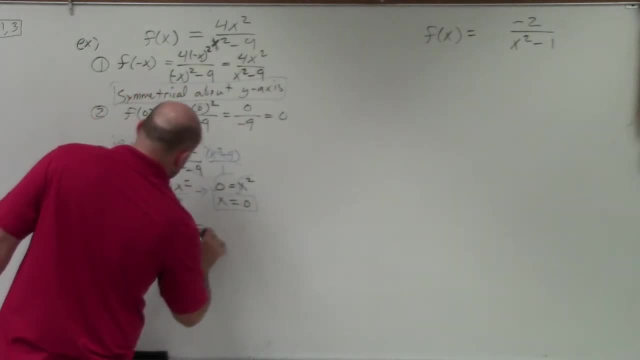 to set my denominator and set it equal to 0.. So I say: x squared minus 9 equals 0.. Now I just go ahead and solve. So I add 9 to both sides, I'm left with x squared equals 9.. Take: 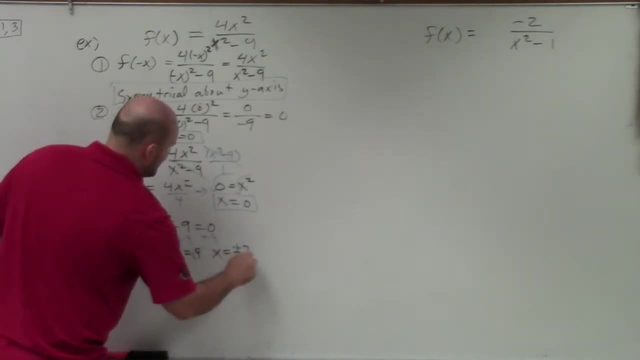 the square root. Take the square root: x equals plus or minus 3.. Remember, when you're introducing the square root to solve you've got to take the positive and the negative values. Last one, Number five, is going to be the horizontal asymptotes. Remember the horizontal asymptote. 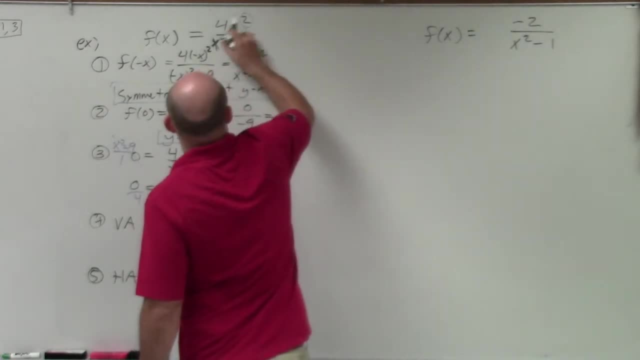 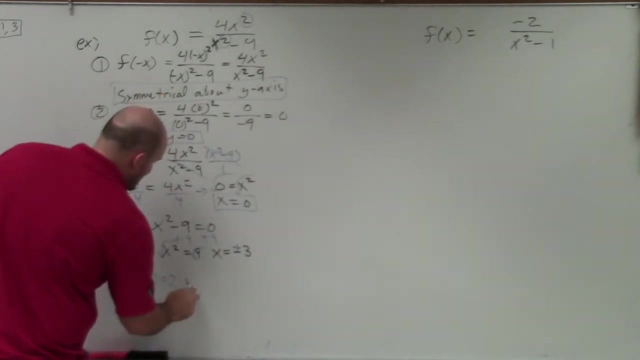 we need to look at the degrees of our function. So we have 2 and 2. They're exactly the same, So 2 equals 2.. So when the degrees are exactly the same, you take: The horizontal asymptote: is a over b, which is the coefficients. Well, here I have x, e squared over b. So what does? that equal? Well, you get plus and minus 3.. And that's the horizontal asymptote of the calculation, right? Well, you get plus and minus 3.. So how do you do that? You take the horizontal asymptote of the equation, So you take the 2 over b, So 2 equals 2 plus 2 equals 2.. So what do you do with this? 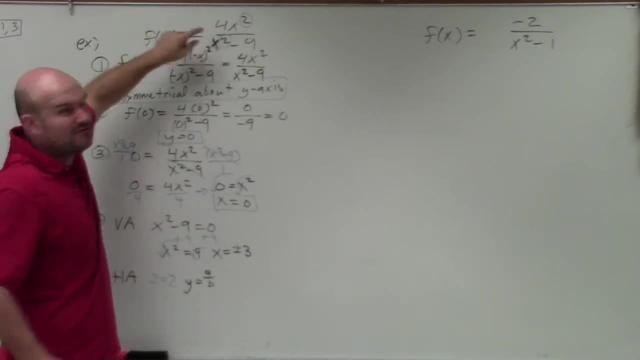 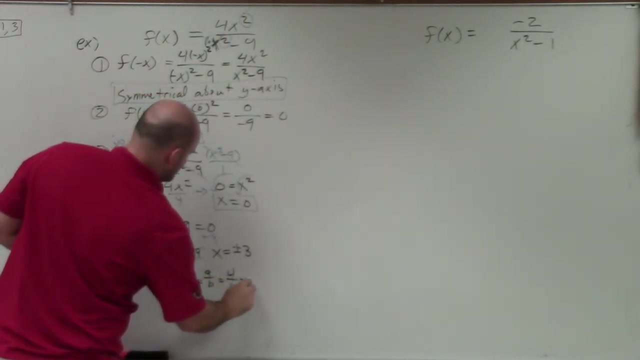 Here I have: 4 is the coefficient of x squared. And then, what's the coefficient of x squared? That's going to be 1.. So I basically have 4 over 1, which is just 4.. So I'll write that as so I have, and y equals 4.. 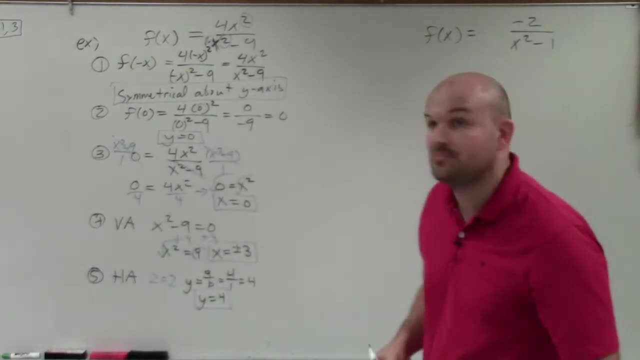 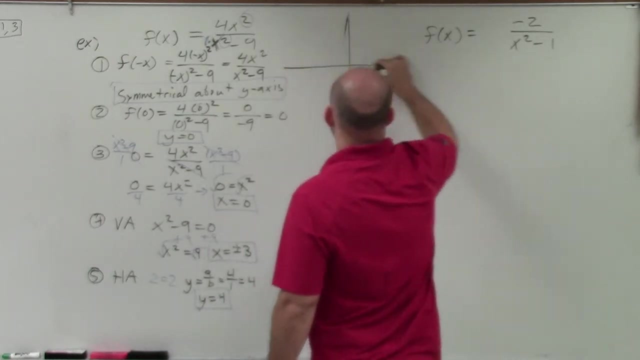 OK. so now, before we go on and get a little bit farther, let's go ahead and plot the information that we have. So I'm at positive 3 and negative 3.. 1,, 2, 3.. OK, those are going to be asymptotes. 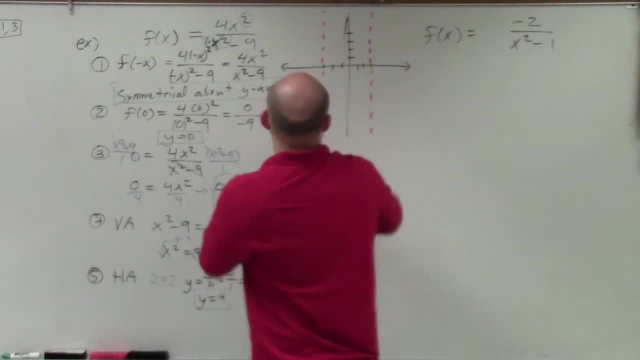 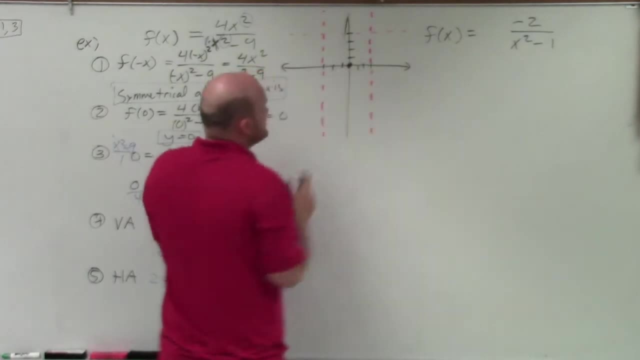 And then I have a horizontal asymptote at 4.. 1,, 2,, 3,, 4.. And I have an x and a y intercept at 0.. Now the reason why, again, this is so important is because, rather than just randomly choosing numbers, 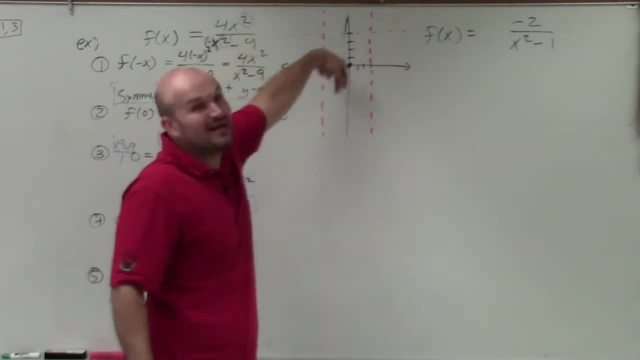 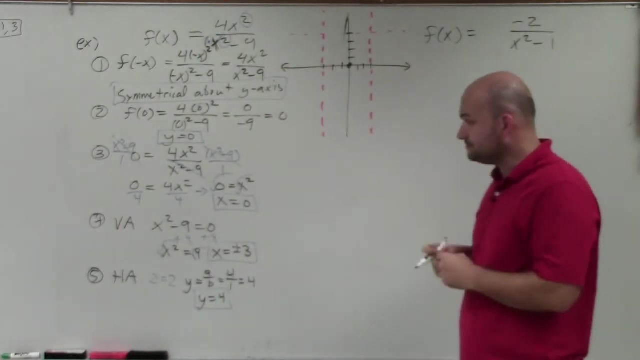 to plug in for your function. I know that I'm going to have to choose values to the left and to the right of every vertical asymptote, But since I have symmetry about the y-axis, I can just focus on one side and then reflect it over. 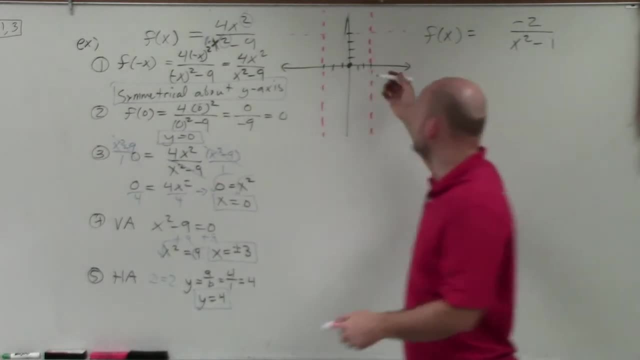 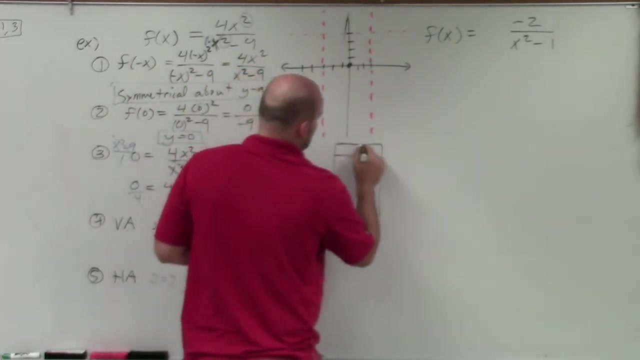 So that's exactly what I'm going to do. So I'm going to choose two points to the left and to the right, And basically kind of think of this again if you're going to create a table of values, Just like if you were going to graph x and y. 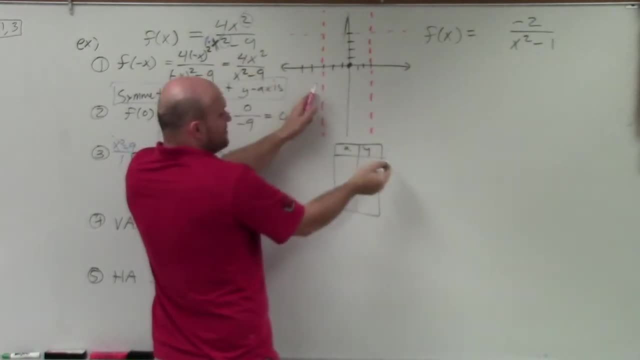 We know if you plugged in negative 3 into this function, you'd get 0. That would be undefined. so that's an asymptote. But so we're going to want to figure out that's negative 3.. We want to figure out the values for negative 5.. 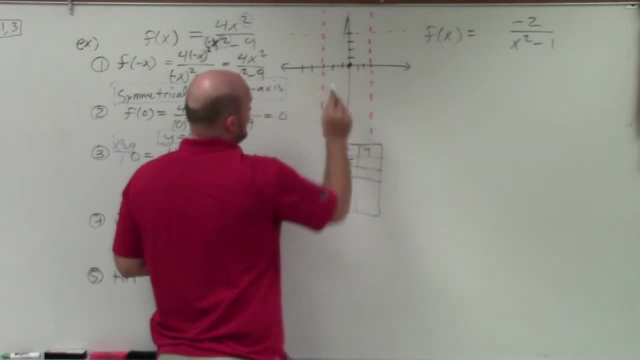 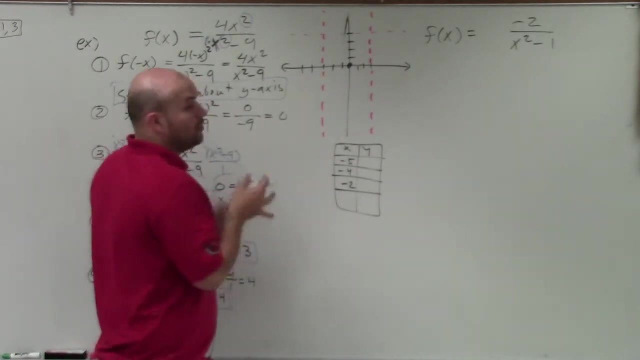 We want to figure out the values for negative 4. And then I'm going to pick the value for negative 2. And then we're just going to plug those in. So how do you figure out what those values are? Well, you plug in the x value in for x, and then find y. 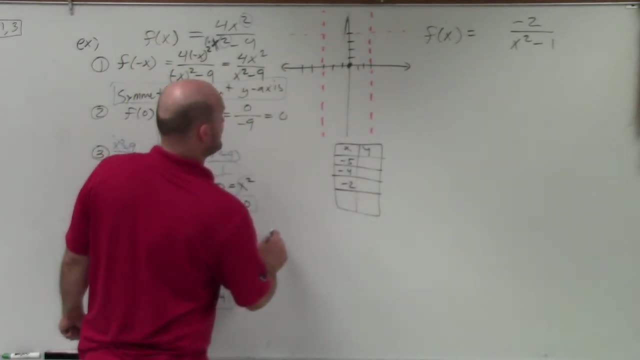 or what f of x is. So I'm going to solve for f of negative 5, f of negative 4, and f of negative 2.. OK, So again, remember, ladies and gentlemen, when you're doing this, basically this: 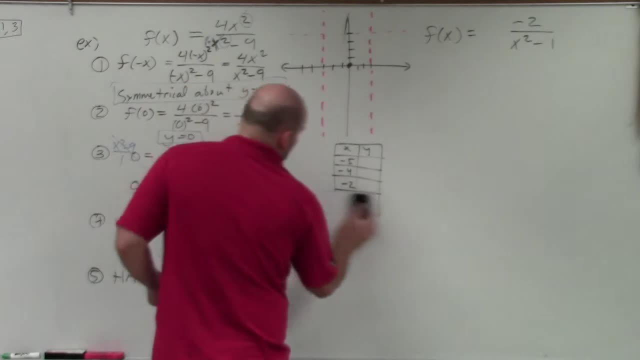 is just like me using a table of values, plugging them in, But I'm using function notation to represent that. Now I'm not going to actually show myself plugging them in, because I did that before And it takes a little long time. 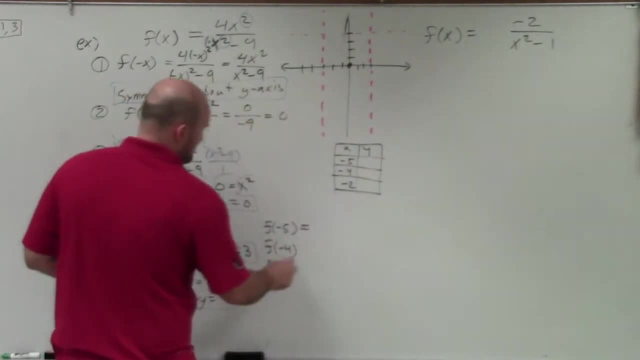 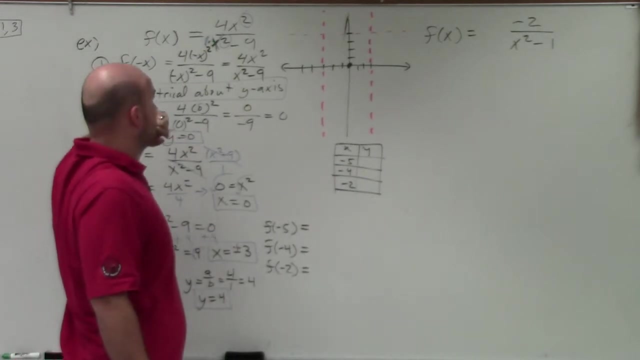 And I want to speed this apart, So I am going to say it out loud and show some of my work here to help you out with that. So if I plug in negative 5, I have negative 5. squared is going to be 25.. 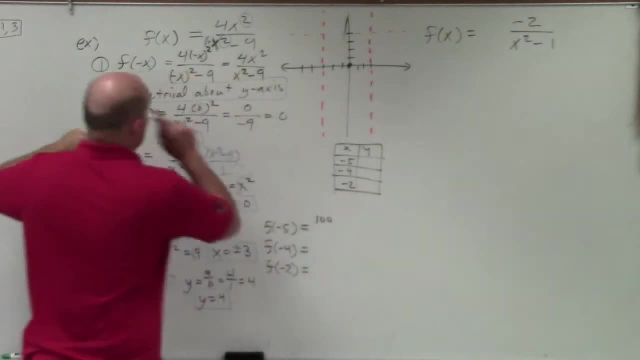 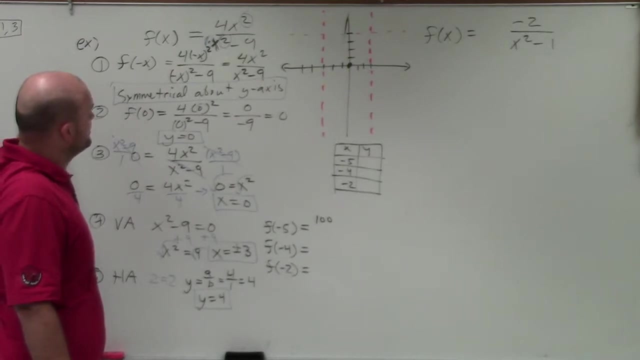 25 times 4 is 100. And then 100. Then a negative 5 squared is going to be 25.. 25 minus 9 is going to be 16.. So let's just do 600 divided by 16.. 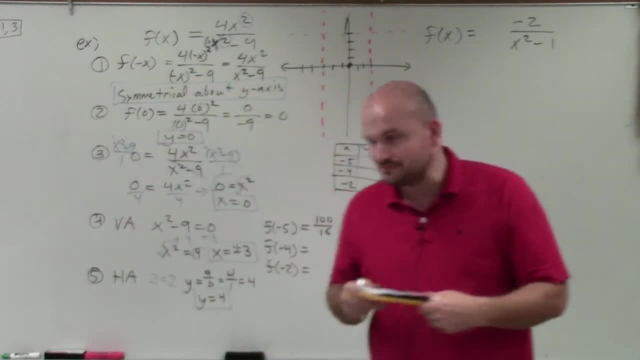 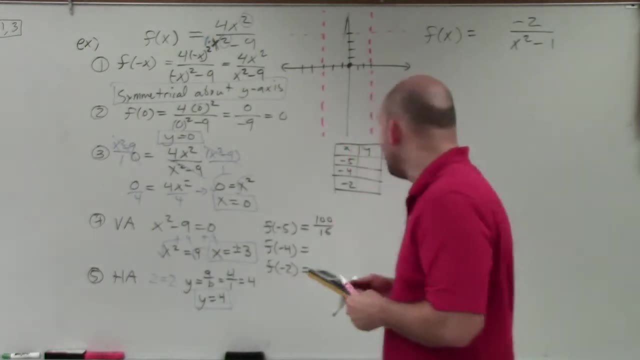 Now, the other thing to remember is when you're dealing with decimals or when you're dealing with graphing. I always like to stay away from decimals. I always like to keep with fractions. But it's very important. We're just graphing. 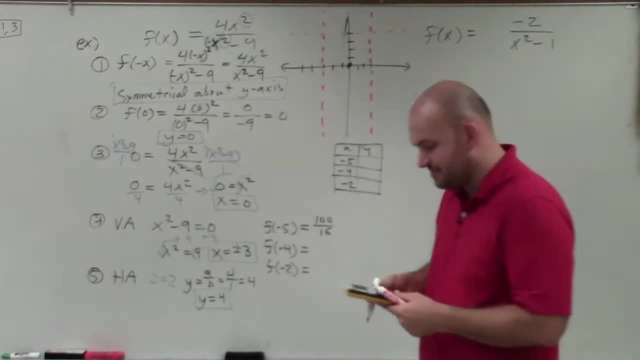 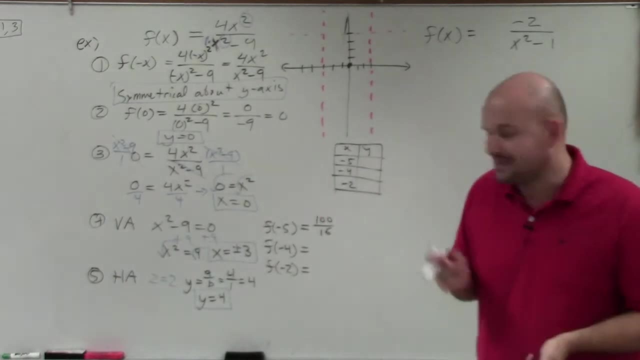 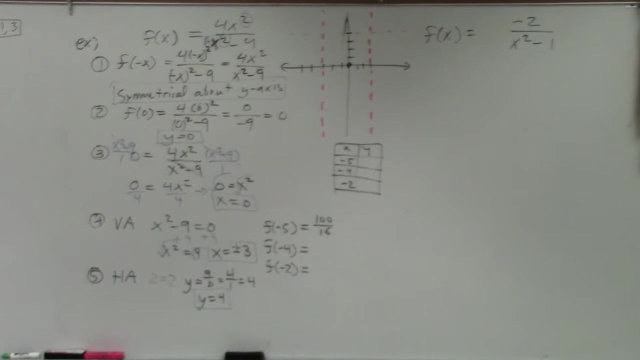 We're just trying to find approximate values, So getting the exact value is OK not to always have, because we're just going to be plotting them And I don't know why my calculator won't turn on, So I'll go back to little grade here. 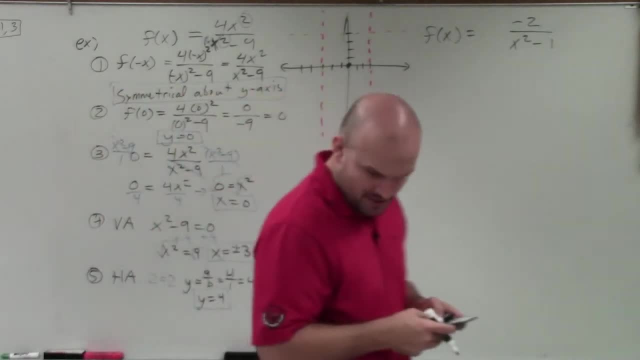 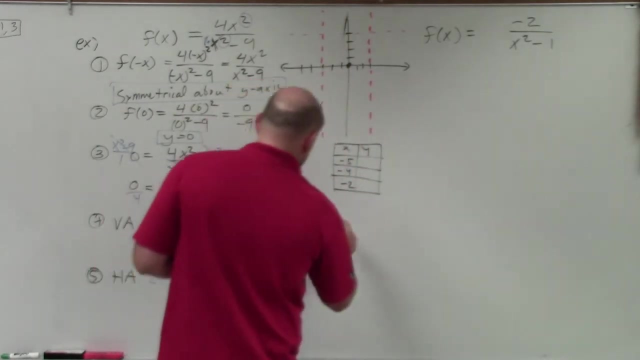 And pick one of these fun ones up, And I just want to make sure I have the right answer. So 100.. Of course this one doesn't work. Divided by 16. What the heck? 6.25.. So I have 6.25. 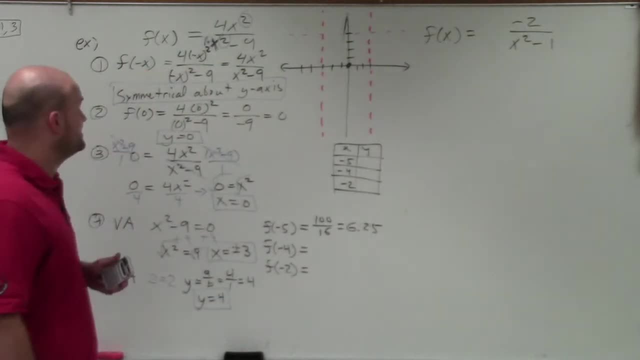 Let's do negative 4.. Negative 4 squared is positive: 16.. Positive 16 times 4 is going to be 64. And then negative 4 squared is 16.. 16 minus 9 is 7.. So let's do 64.. 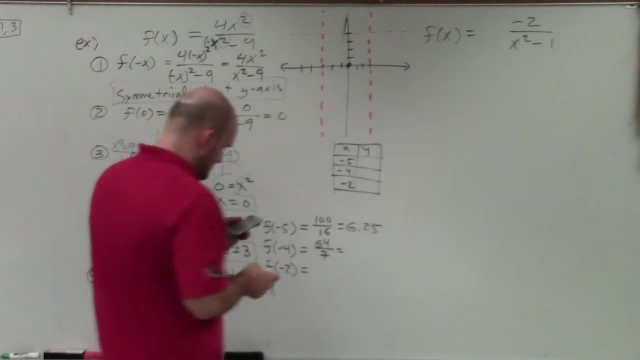 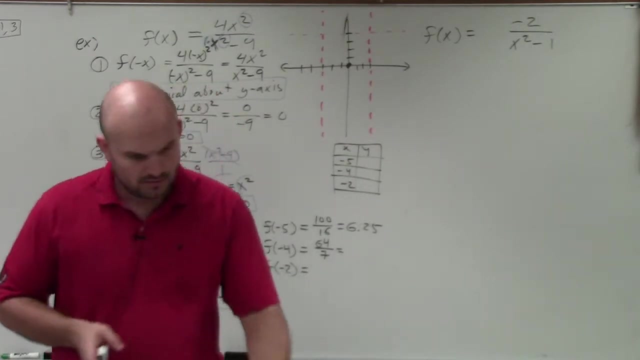 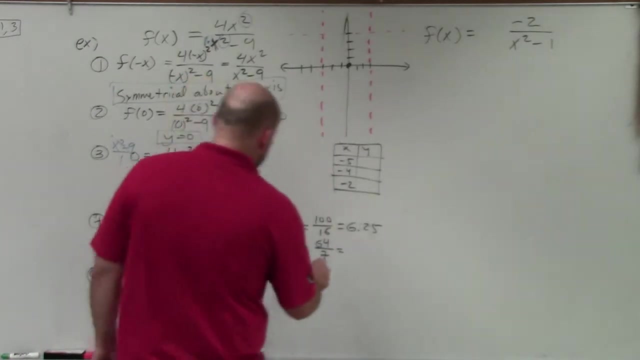 64 divided by 7.. And that gives me 64 divided by 7.. What the heck is that? What the heck is that? OK, Now this one turns on: 64 divided by 7 is 9.14.. So I'll just round that to 9.1.. 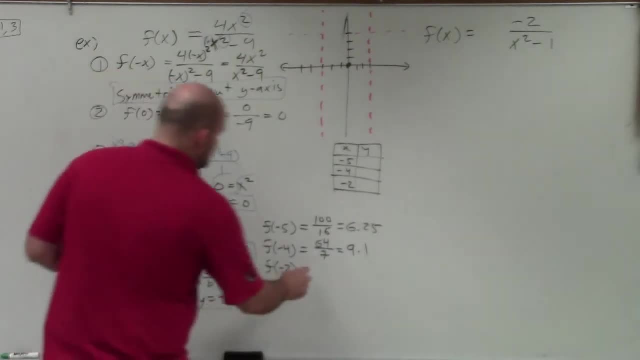 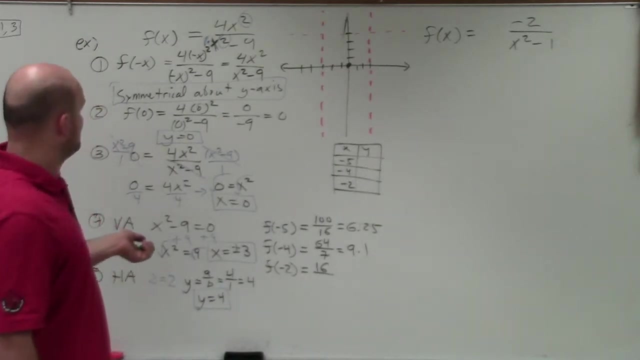 And then at negative 2. Negative 2 is positive 4. 4 times 4 is 16.. And then negative 4,, so that's 16.. So then that's negative. Negative 2 is 4.. 4 minus 9 is going to be negative 5.. 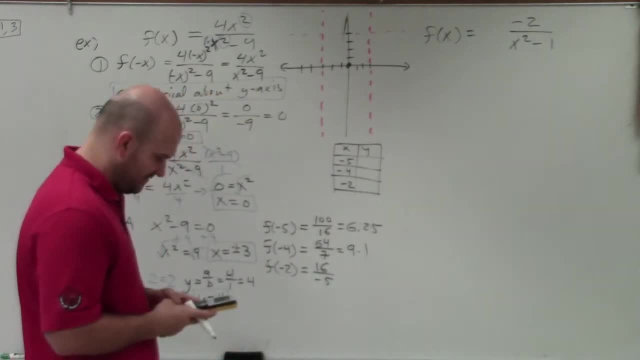 So let's go and reduce that Divided by negative 5. I guess I probably could have done that in my head. Negative 3.2.. OK, So again we can use symmetry. So we can use just half of this. 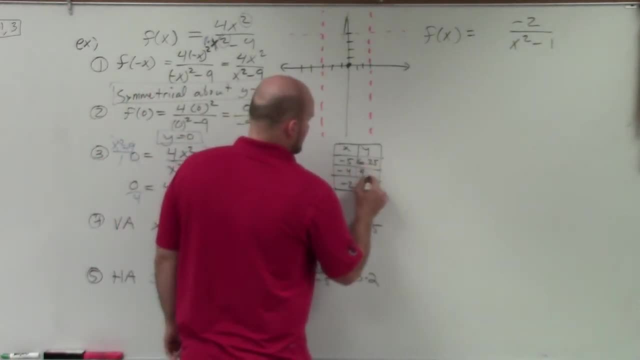 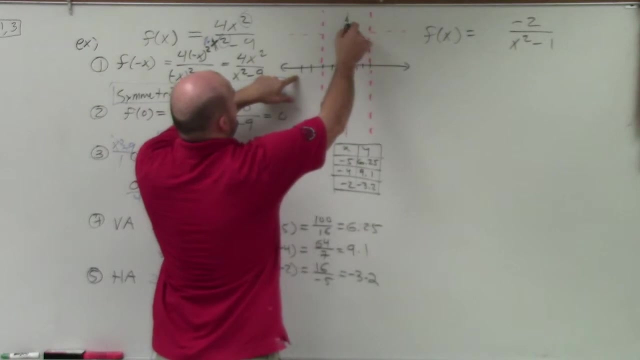 So basically these are coordinate points 6.25.. 9.1.. And negative 3.2.. So let's plot the points At negative 5, I'm at 9.1.. 1,, 2, 3, 4,, 5,, 6,, 7,, 8,, 9.. 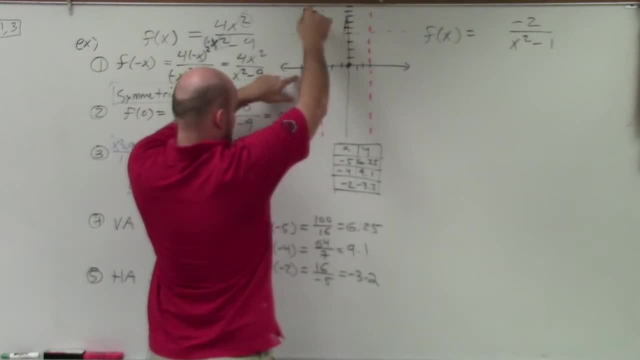 Way up there. Oh No, I'm sorry. Negative 5,, I'm at 6.25.. At negative 4,, I'm at 9.1.. And then over here at negative 2,, I'm at negative 3.2.. 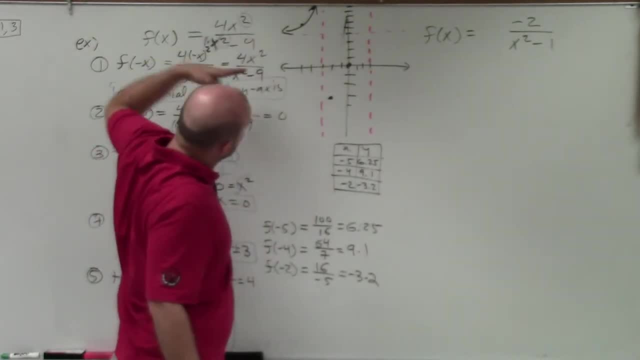 So again for my graph, Remember I connected them. I want them to approach the asymptote. So it's going to show like a little hyperbola. It's going to approach the vertical asymptote And then it has to approach the asymptote. 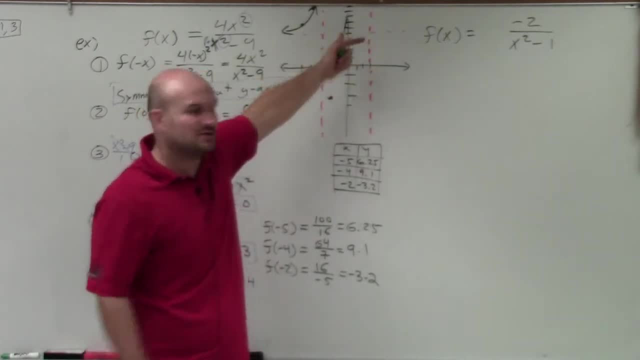 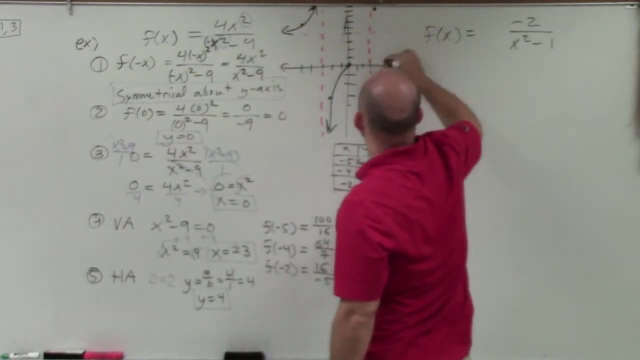 Here I've got to connect these points, But they can't go up because then it's going to kind of go to a dead end. So it's going to have to look like this: So now, if I just reflect these points, 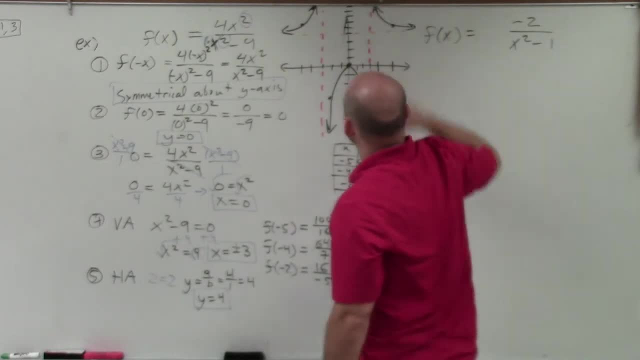 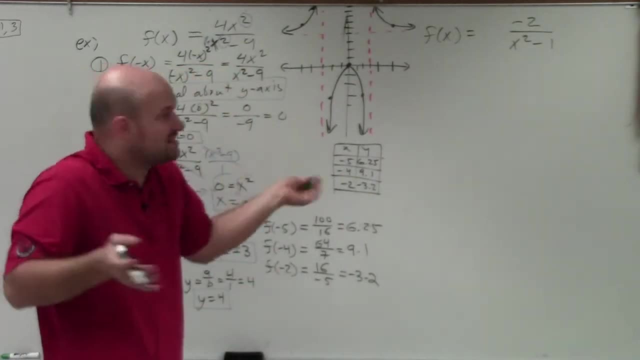 then I can just use symmetry now to make my graph. Isn't that nice? Isn't symmetry nice? So I only had to use one, two, three points instead of finding six points. OK. So now let's go into the next example here. 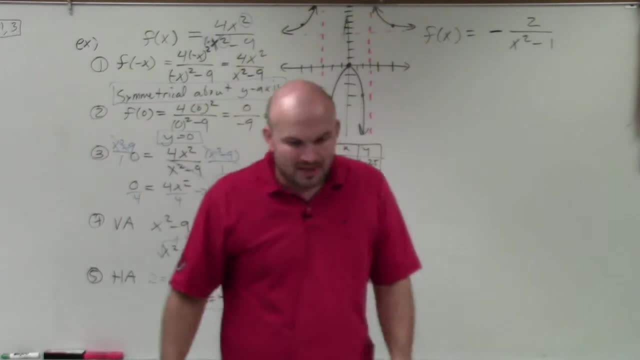 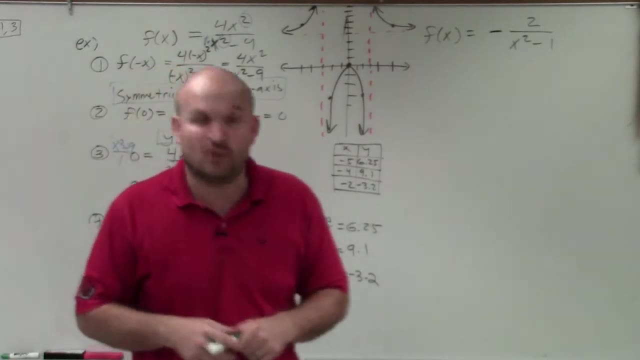 And actually I wrote this wrong because I made a mistake on this video So I had to recreate it, So I didn't actually. So the actual original problem is: f of x equals negative 2 divided by x squared minus 1.. 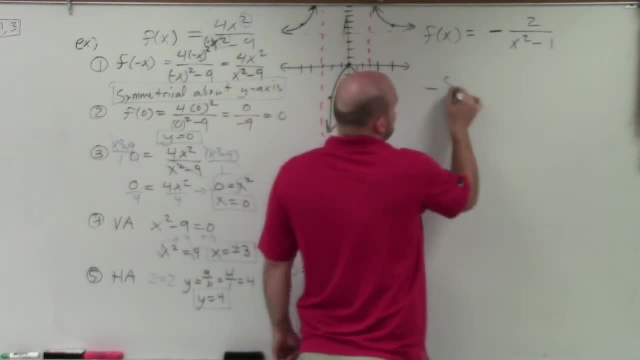 Now the reason why I had that 2 up there instead of because what I was telling in my first video was: if you have a negative 8 over 4, that's the same thing as negative 8 over 4,, which is equivalent to 8 over 4.. 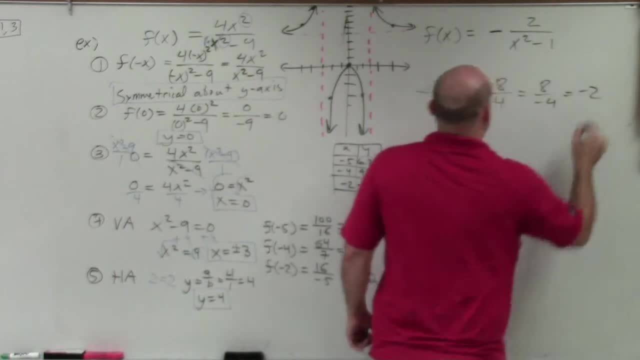 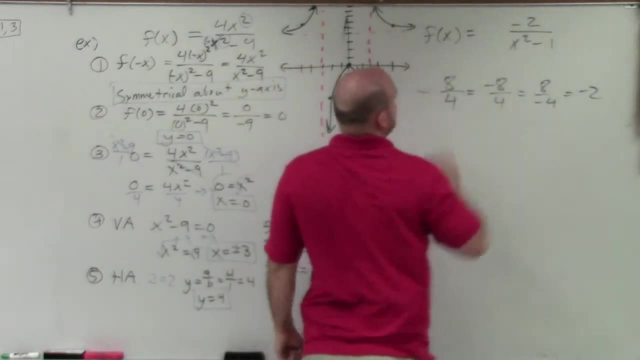 It's equivalent to 8 over negative 4, which all equal negative 2.. So when you have a negative in front of a fraction, just put the negative in the numerator or in the denominator. So what I did was I said I'm going to put it in the numerator. 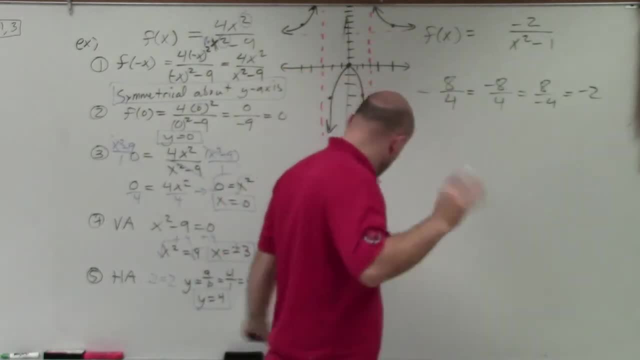 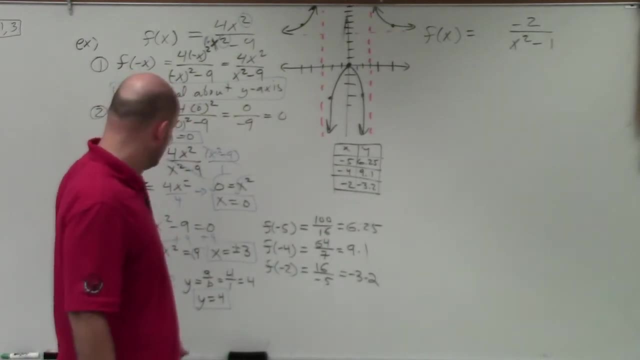 Because I'd rather put it in the numerator than put it in the denominator and have to negate a binomial, which would not be fun. It's not really hard, It's just extra work, OK, So I'm kind of running out of space here. 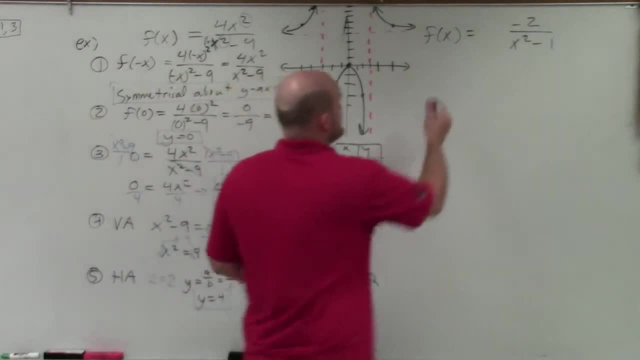 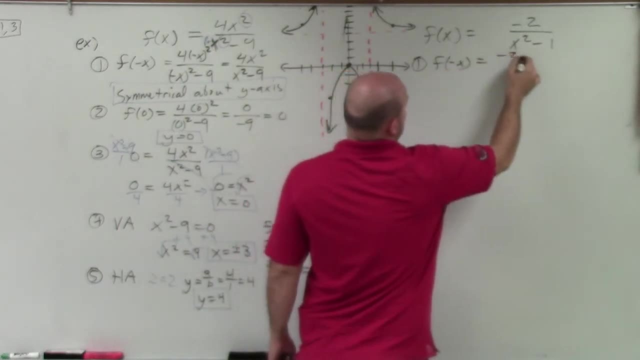 So I'm going to try to do my best to really scrunch everything in. So the first thing I need to do, step number one, is again find the symmetry f of negative x. So I get negative 2 divided by negative x, squared minus 1.. 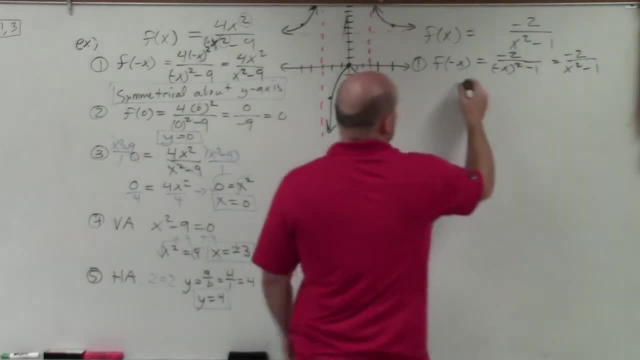 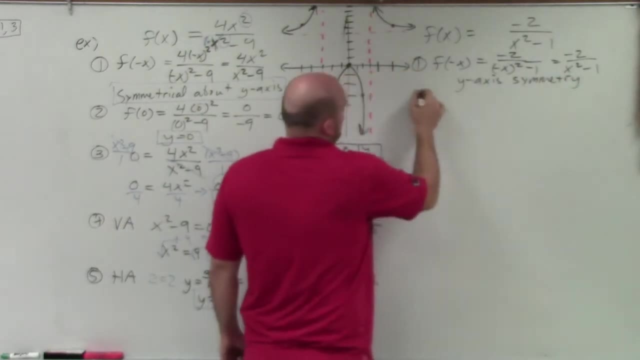 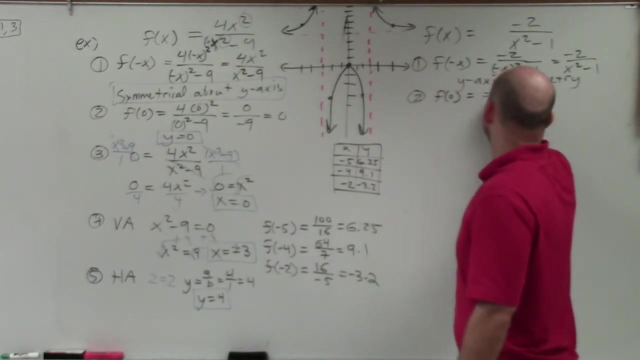 Well, that gives me negative 2 divided by x, squared minus 1.. So again we have y-axis symmetry. Sweet Number two: we want to go ahead and find the y-intercept. So I do: f of 0 equals negative 2 divided by 0, squared minus 1.. 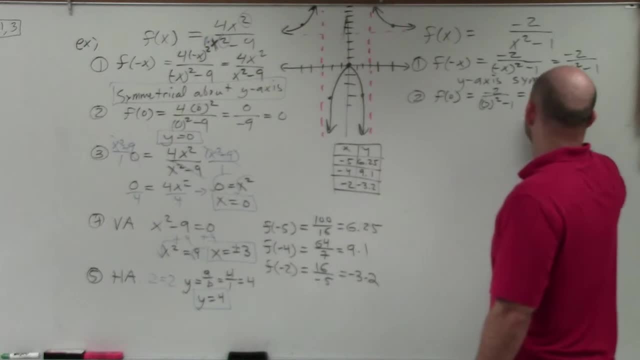 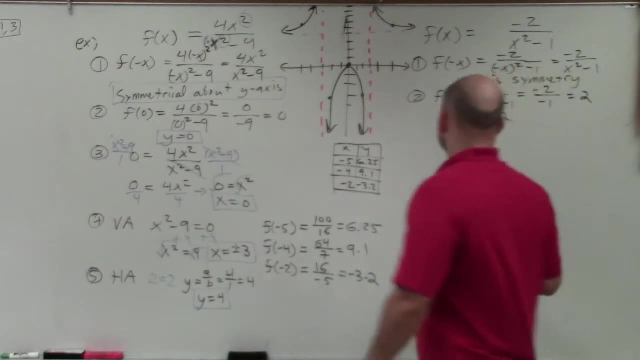 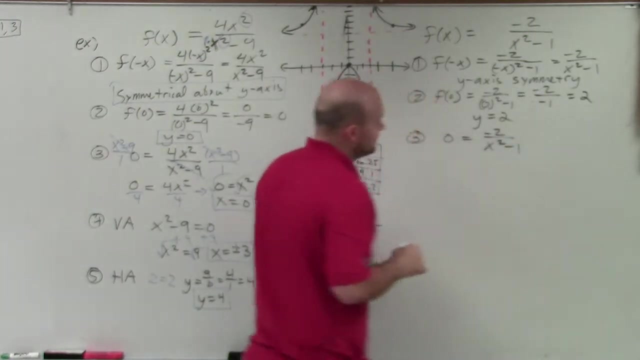 So that becomes negative 2. Divided by 0 minus 1, which is negative, 1, which equals positive 2. So my y-axis is: y equals 2.. Then I find the x-axis: 0 equals negative 2 divided by x squared minus 1.. 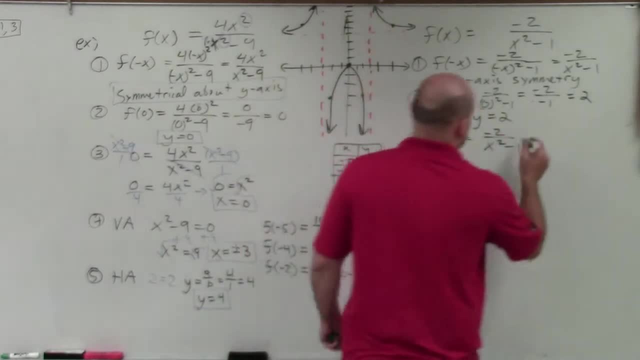 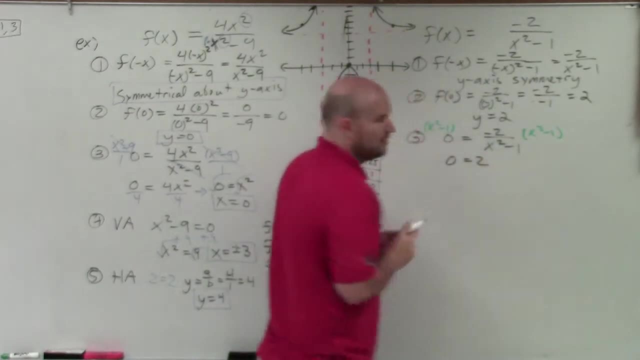 So here, when I multiply, this one gives me a very nice one. I like this. So I multiply by x, squared minus 1 on both sides, And what I'm left with is 0 equals 2.. Well, 0 does not equal 2.. 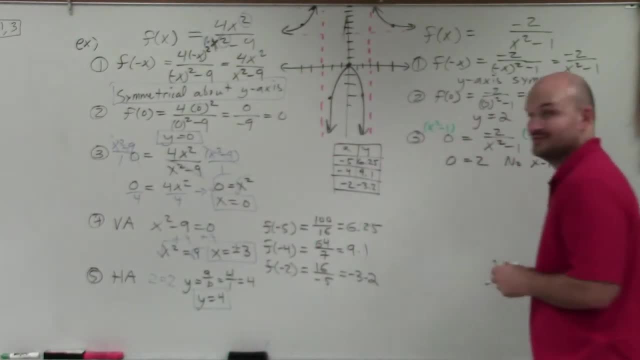 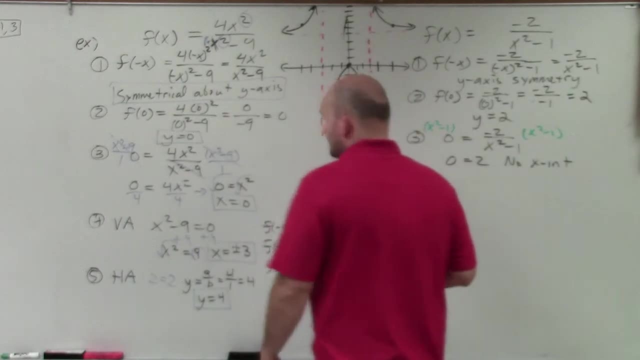 So, guess what? There's no x-intercept, So the graph is never going to cross the x-axis, which is possible, And that's cool. Step number four: vertical asymptote. So in this case we're going to do: x squared minus 1 equals 0.. 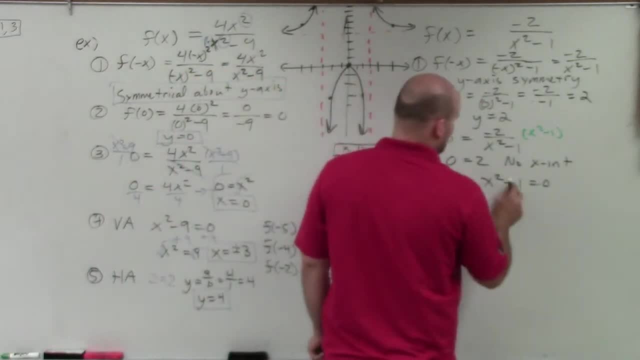 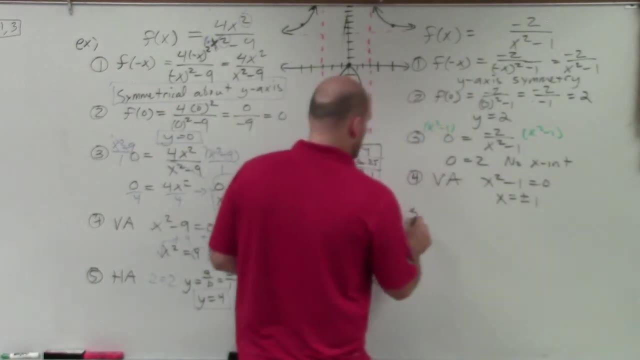 You take your denominator, set it equal to 0.. Here I go ahead and solve: Add 1 to both sides, take the square root, Make sure you include the positive and the negative. x equals plus or minus 1.. Step number five: horizontal asymptote. 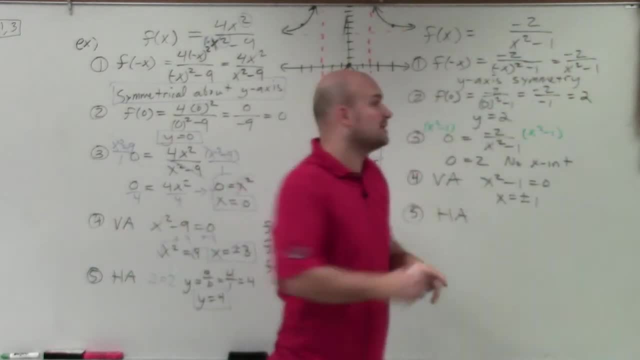 Now again, We look at the degrees. Now this one. you say, well, there's no degree in the numerator. Well, yes, there is actually. You can actually write x to the 0, because x raised to the 0 is equal to 1.. 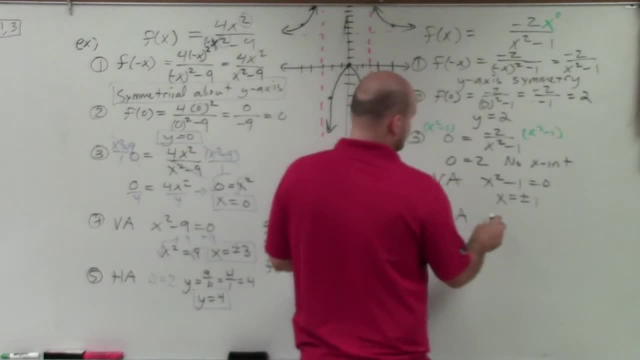 And negative 2 times 1 is 1.. So therefore we have 0 and 1. And obviously 1 is greater than 0. So whenever the degree in your denominator is larger than the degree in your numerator, we have an asymptote at y is equal to 0.. 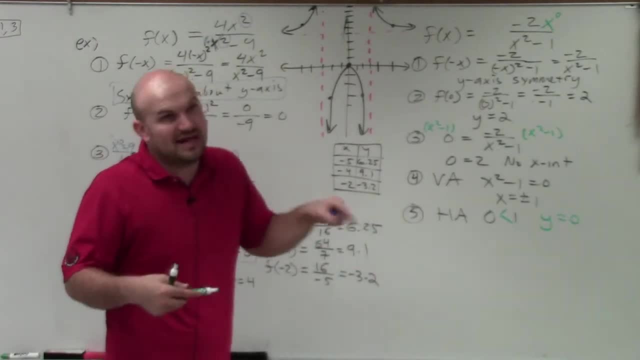 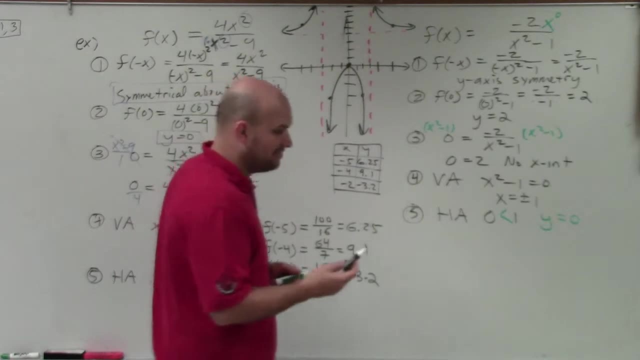 That's why the graph doesn't cross. Now there's times where you're going to have a horizontal asymptote and the graph will cross, But in this example it's not going to cross at 0.. So now we need to go ahead and plot our information. 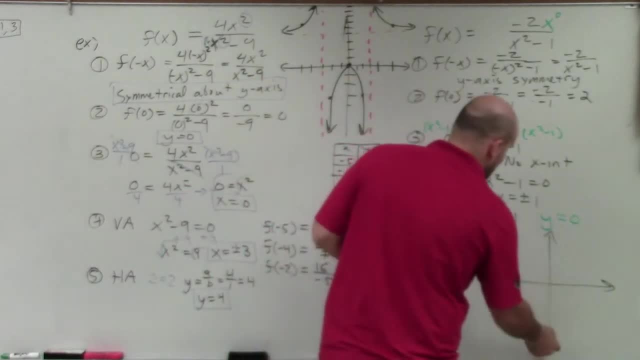 Now again, remember: we have symmetry, So we only need to focus symmetry on one side of the graph. But let's plot what we have for your first. First of all, we know that the y-intercept is going to be at y equals 2.. 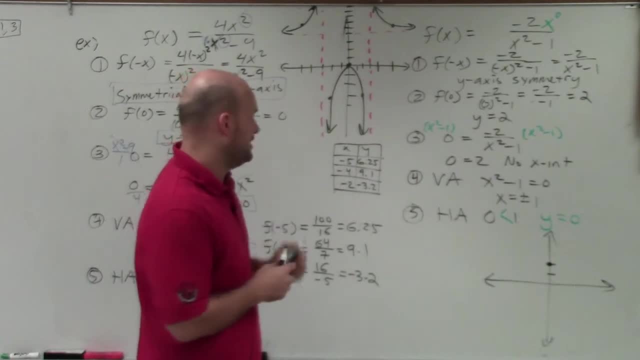 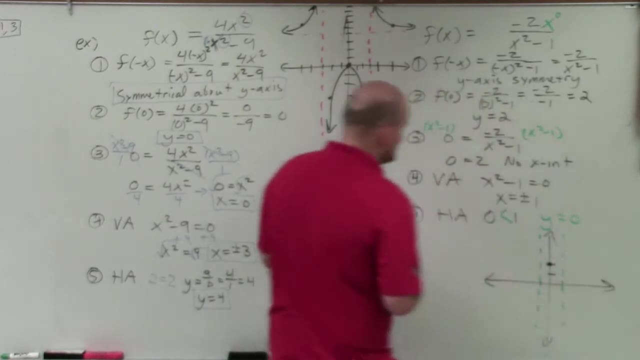 We know that the x-intercept does not exist. We have vertical asymptotes at positive 1 and at negative 1.. Oh, this is step number 6,, by the way, is plotting the information. And a horizontal asymptote at y equals 0.. 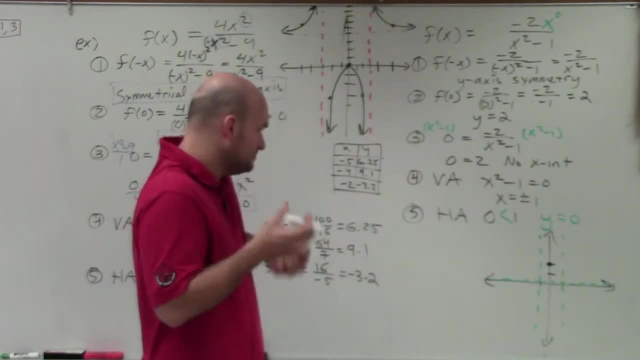 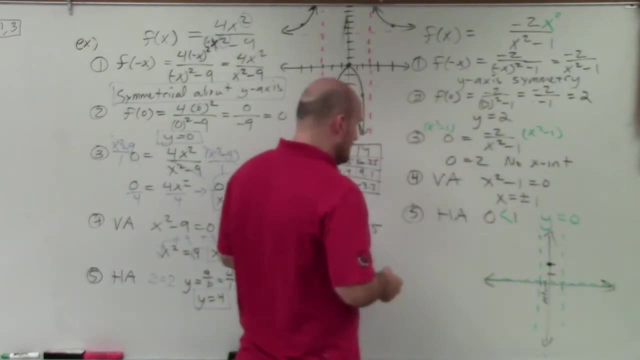 So now I need to determine some points And again I'm just going to choose points to the left and to the right. So I have negative 1.. I'm going to plug 1 and 1 half as a point. I'm going to pick 1 half. 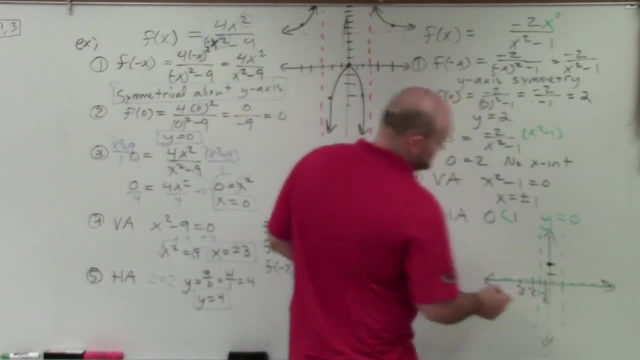 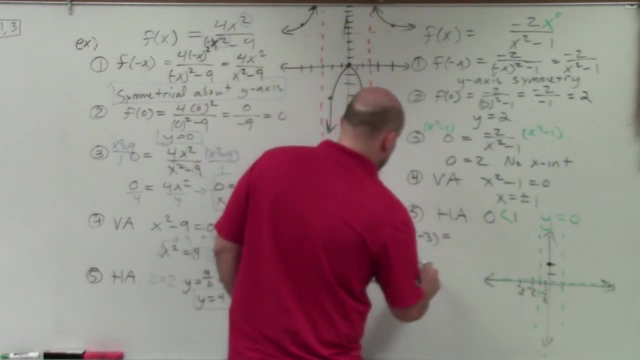 And then that's negative 1, so negative 2 and negative 3.. So those are going to be your three points I'm going to want to figure out. So I'm going to do f of negative 3.. I'm going to do f of negative 2.. 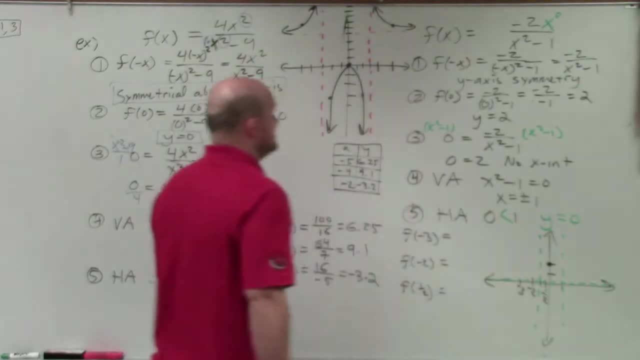 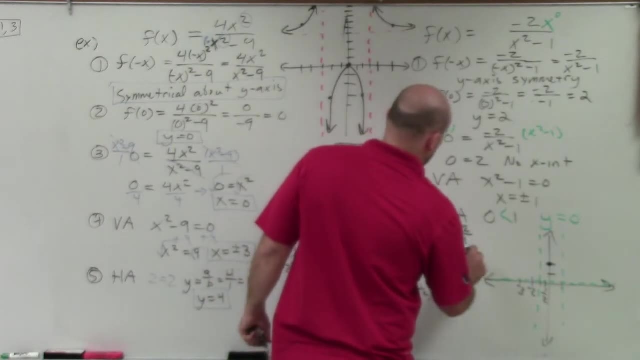 And I'm going to do f of 1 half, So let's see if we can plug them in. So I have negative 2.. So negative 3 squared is 9.. 9 minus 2 is 8.. So I have negative 2 over 8, which equals a negative 1. fourth, 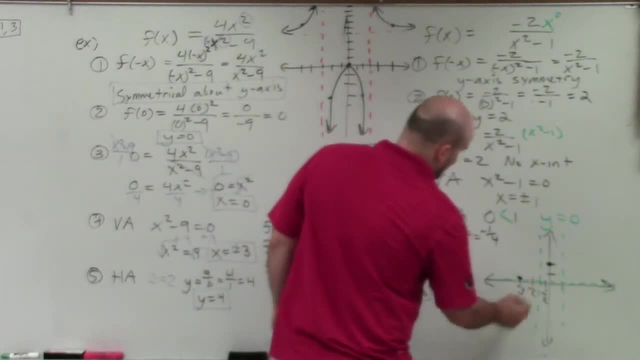 So at negative 3, I'm at negative 1. fourth, which is almost at the asymptote, Let's do negative 2.. Negative 2 squared is positive 4.. Positive 4 minus 1 is 3.. So I have negative 2 over 3.. 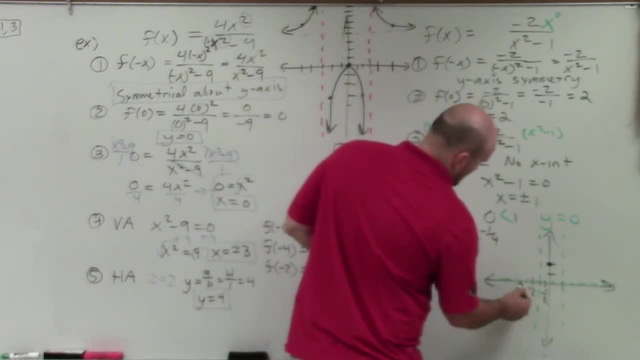 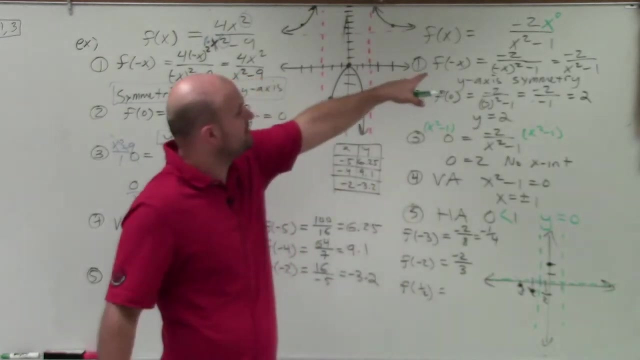 Oh, that's a negative 1 fourth And negative 2 thirds is almost a 1, but it's not quite there. But it's getting there, OK. And then let's do f of 1 half. So 1 half squared is going to be 1 fourth. 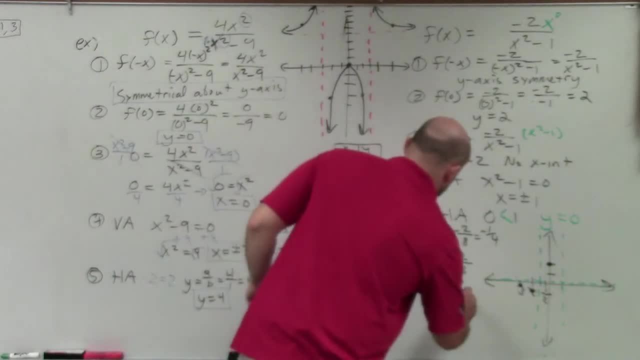 1 fourth minus 1 is going to be a negative 3 fourths. So I have a negative 2 divided by a negative 1 fourth. Oh no, sorry, negative 3 fourths. If you remember in my first video. 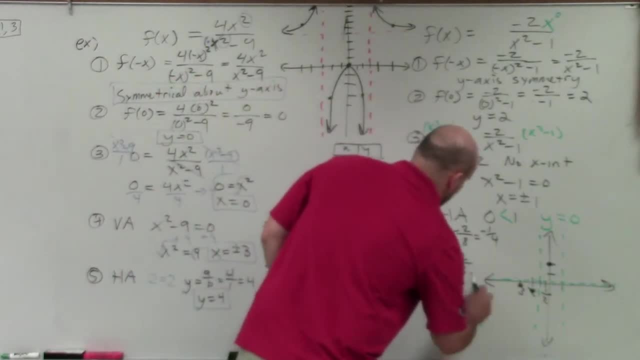 how do you get rid of the fraction in the denominator? Multiply by the reciprocal- OK. How do you multiply negative? OK, That's going to go to positive. So let's just multiply by the negatives. So then that multiplies to give you 1.. 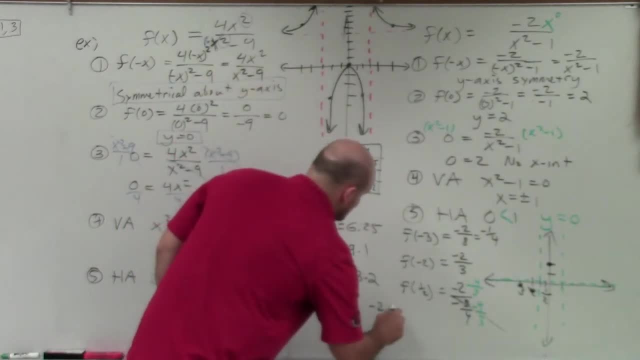 So you're left with a negative 2 times negative- 4 thirds. Negative 2 times negative: 4 thirds. Put the 2 over 1.. Multiply across, You get a positive 8 thirds. So if you remember from last video that was positive: 2.6..